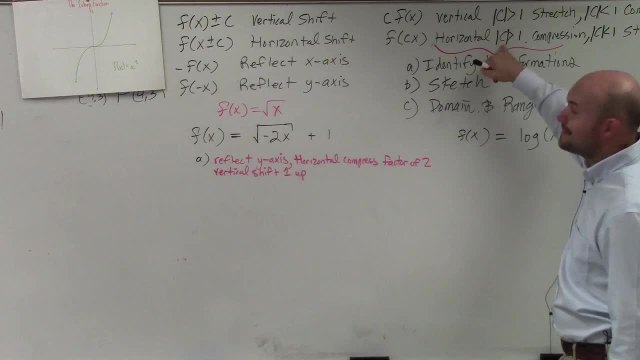 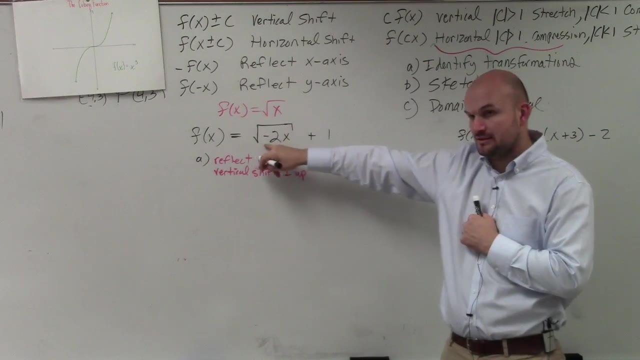 The factor of 2, because that's what I'm multiplying it by And remember it's absolute value of c. So what are you multiplying by your function? Remember c is what you're multiplying by your function. What are you multiplying by Negative 2, but it's the absolute value of. 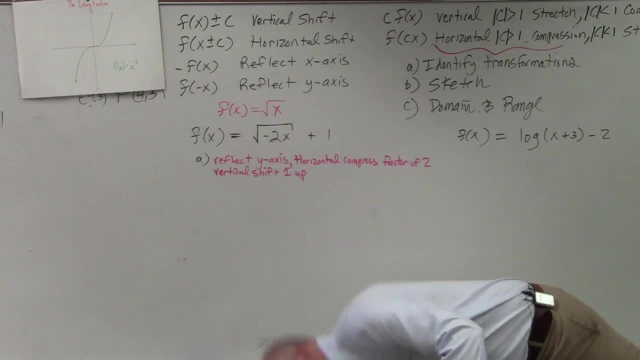 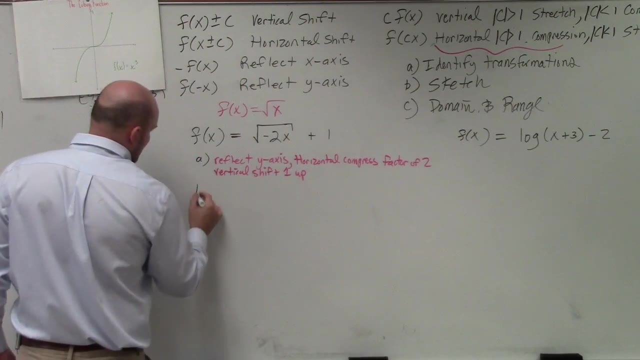 negative 2.. So the absolute value, remember, is the absolute positive distance of that. So absolute value of negative 2 is positive 2.. All right, so now let's get to the graphing portion, And this is why it's important to. 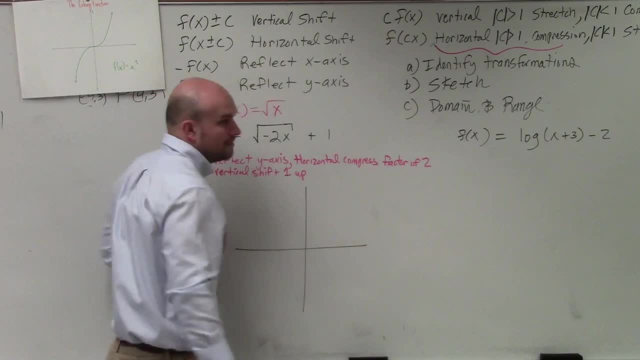 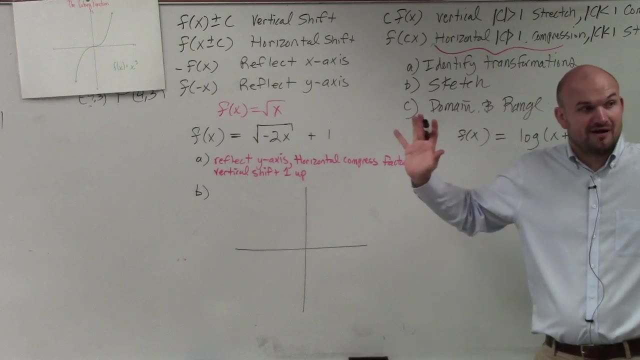 know what the graph looks like, Because if you're going to look at what the graph looks like, we need to remember what square root graph looks like, just the parent graph. It doesn't need to be perfect, But I have this written up there on the board. Oh, graph parent functions right over there. 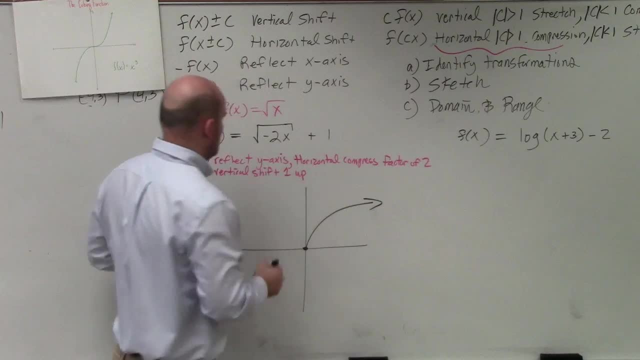 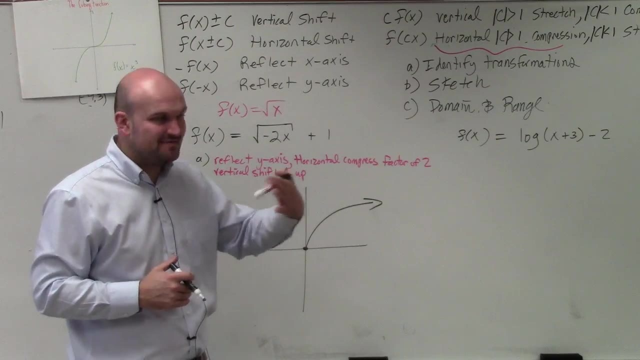 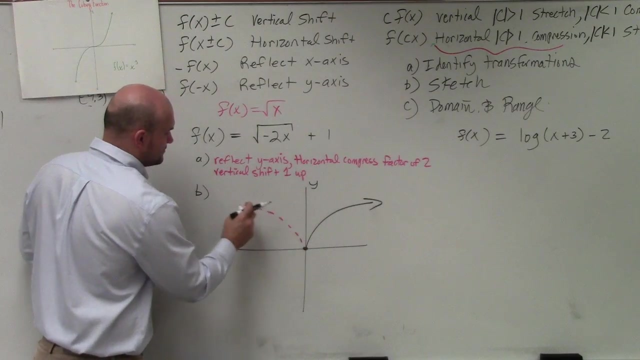 It looks something like this, Right, Something like that. It doesn't even need to be perfect. Now let's apply each transformation individually. I'm going to reflect the y-axis. Here's the y-axis, So my graph looks something like this. now I'll deal with the horizontal compression. last, 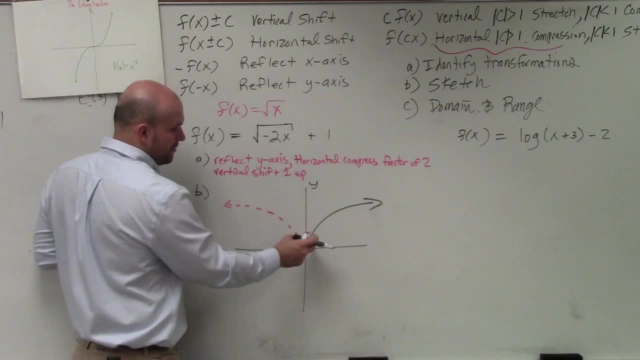 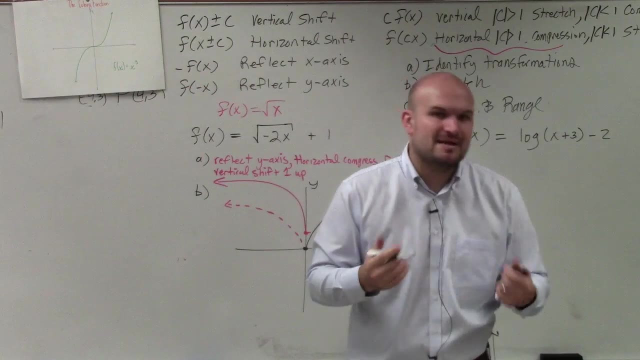 And I have to vertically shift up one. So if originally it was at 0, now it's up 1.. So I'll say: the graph is going to look something like that. Just a little FYI, I am not going to mark you down and say your horizontal compression. 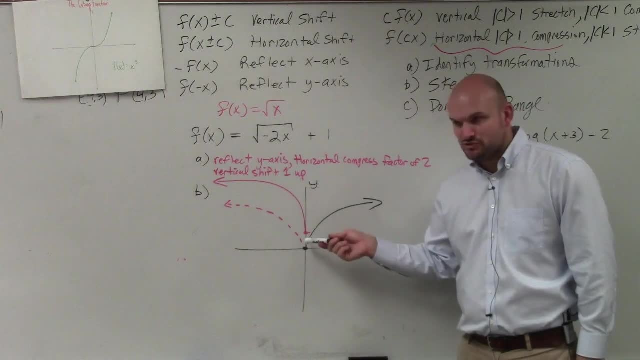 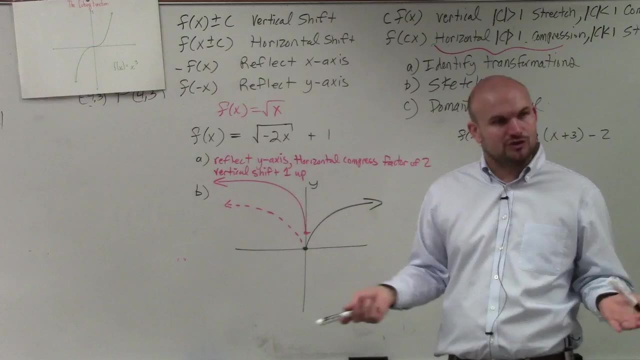 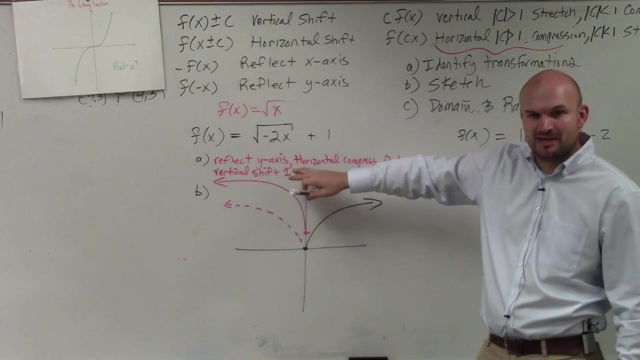 was not good enough. It's easy for me to identify that you shifted the graph up one. It's easy for me to identify if you reflected the y-axis, If you're applying a correct vertical compression or stretch or horizontal compression or stretch, as long as you've noted it in here, for me I'm not. 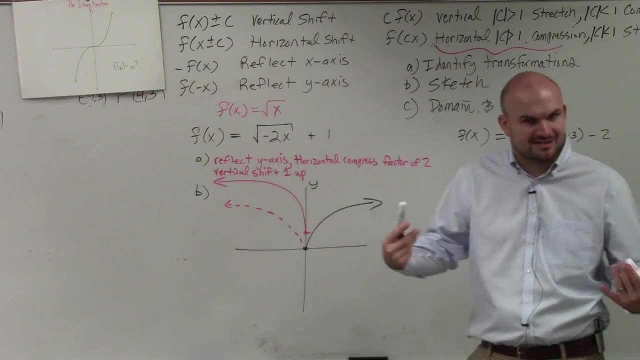 going to say that you didn't do it in your graph, But just be cognizant of it a little bit. And horizontal compression is basically me and your computer. I'm not going to say it's not good enough, It's just that you can see it. I'm not going to say it's wrong, I'm going to 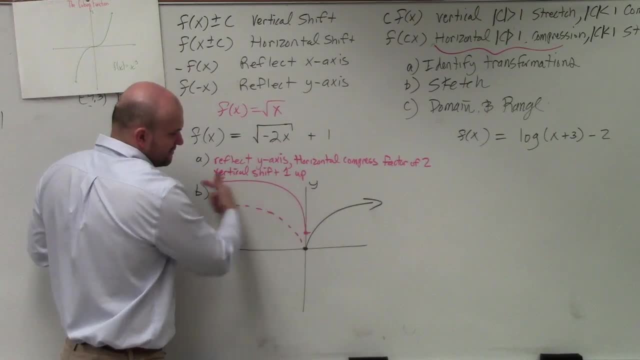 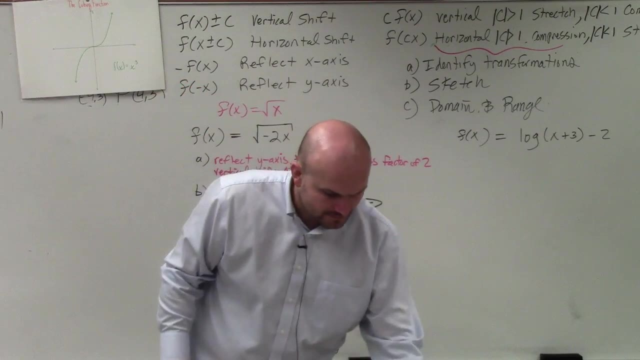 of squishing it right a little bit, so that's why I kind of have a little bit of a sharper curve compared to my paragraph. but again, don't worry about as far as it's catching, you're not gonna be marked down for that. the next thing we